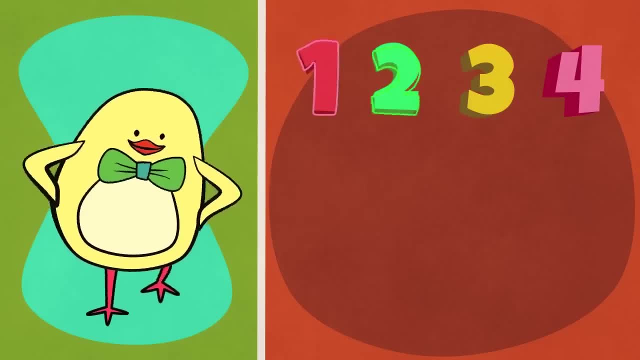 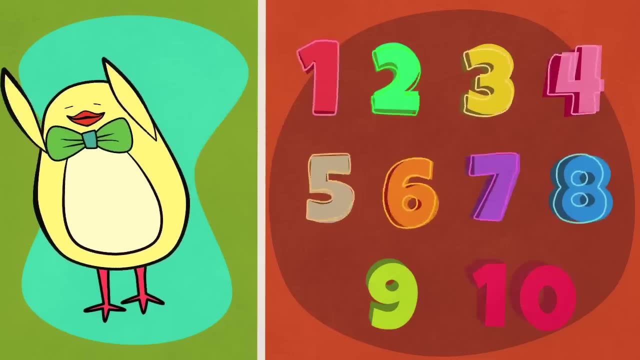 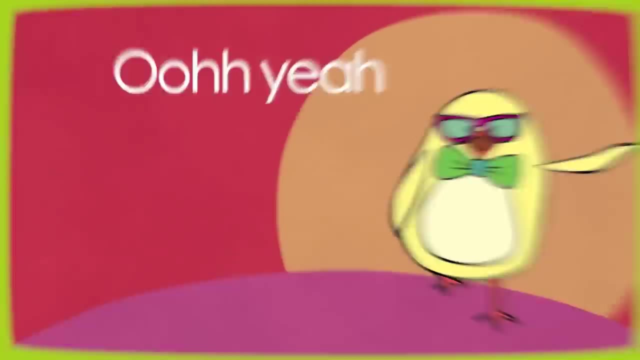 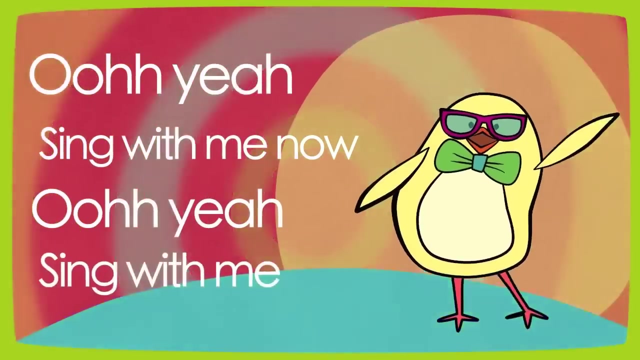 1,, 2,, 3,, 4, 5,, 6,, 7,, 8, 9 and 10. Raise your hands. Boo-yep, Same with me Now. Boo-yep, Same with me. Boo-yep, Same with me. 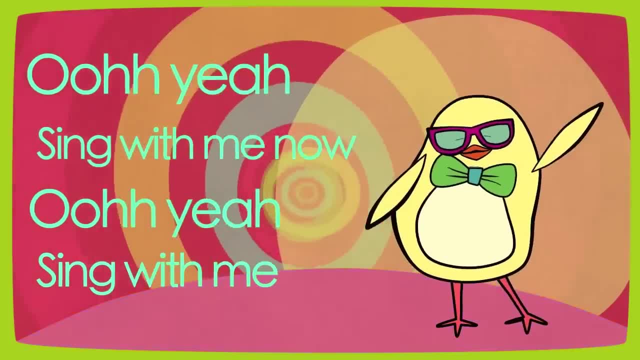 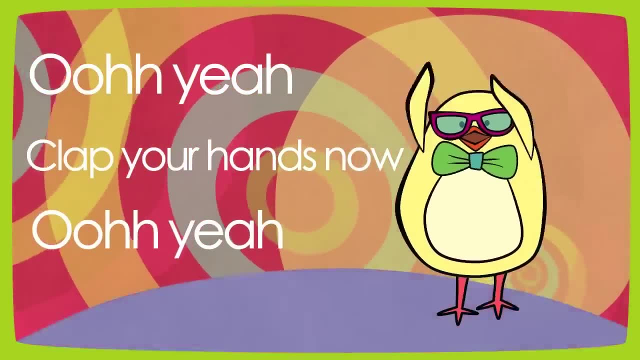 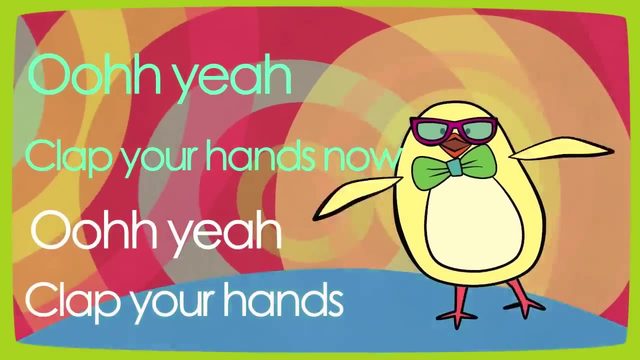 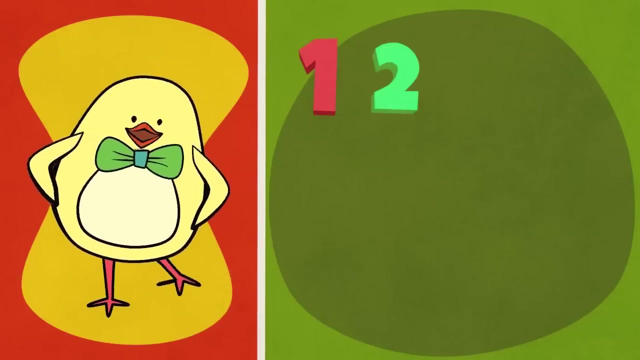 Now: Boo-yep, Same with me. Boo-yep, Clap your hands now. Boo-yep, Clap your hands. Boo-yep, Clap your hands now. Boo-yep, Clap your hands now. 1,, 2,, 3,, 4. 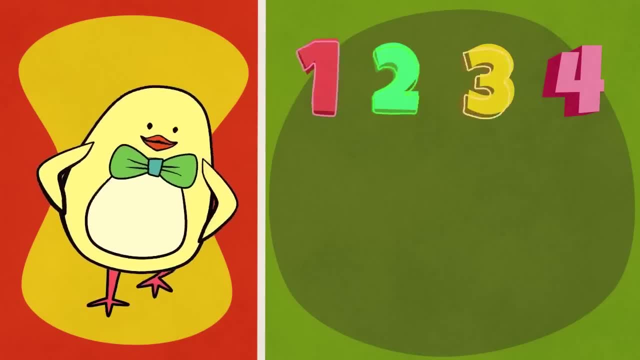 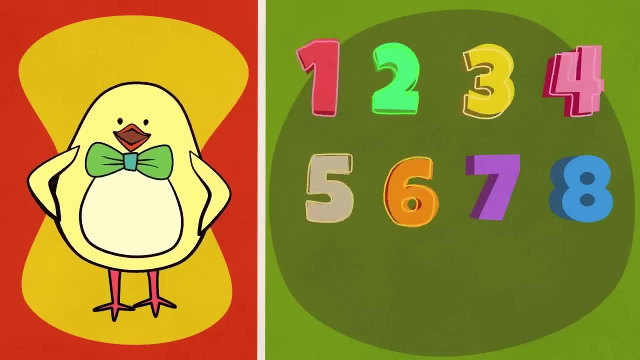 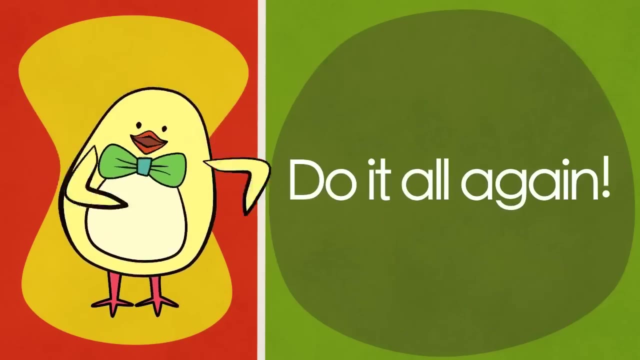 1,, 2,, 3,, 4, 5, 6, 7, 8, 5, 6, 7, 8, 9 and 10, 9 and 10. Do it all again. Do it all again. 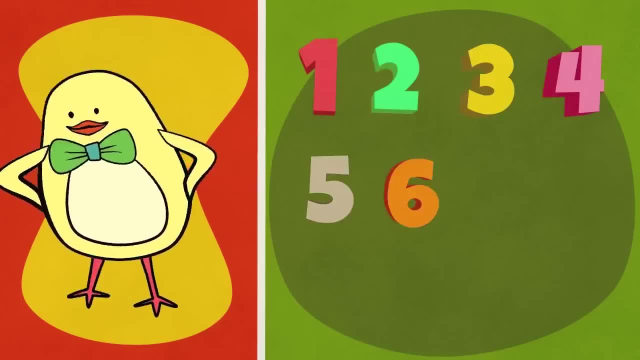 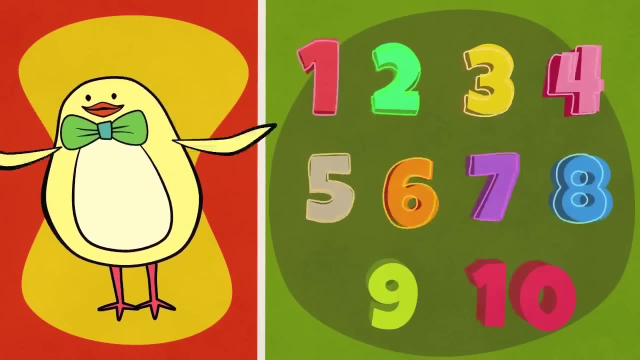 1,, 2,, 3,, 4, 5,, 6,, 7,, 8. 1,, 2,, 3,, 4, 5,, 6,, 7,, 8, 9 and 10. Raise your hands. 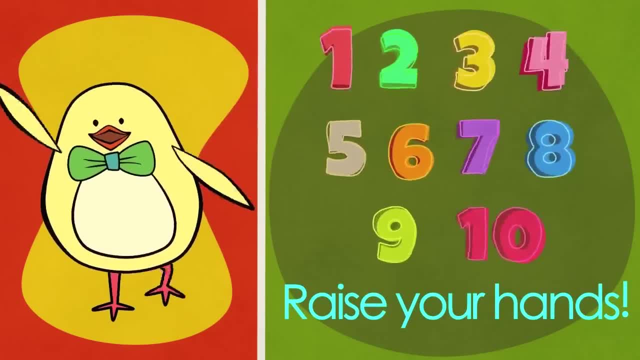 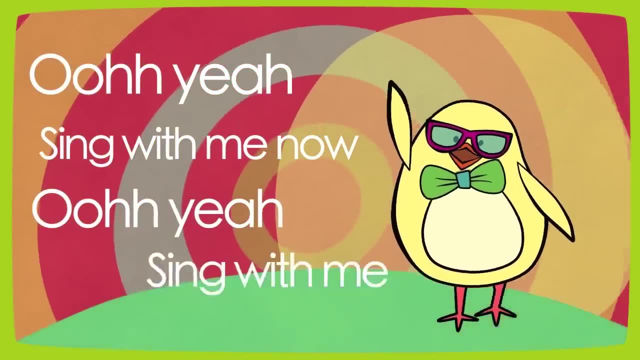 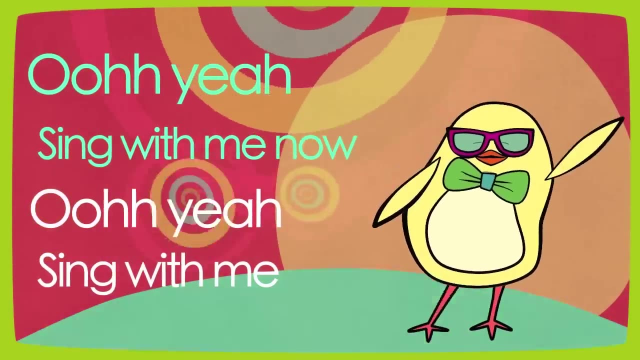 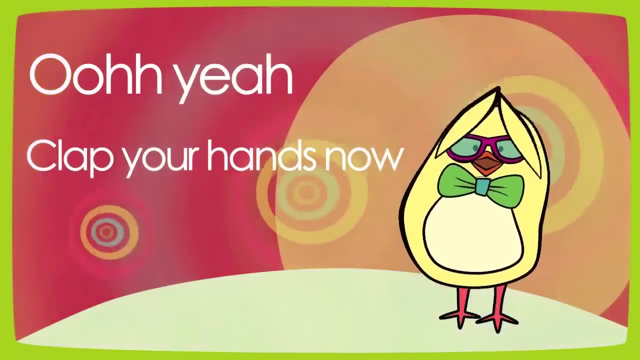 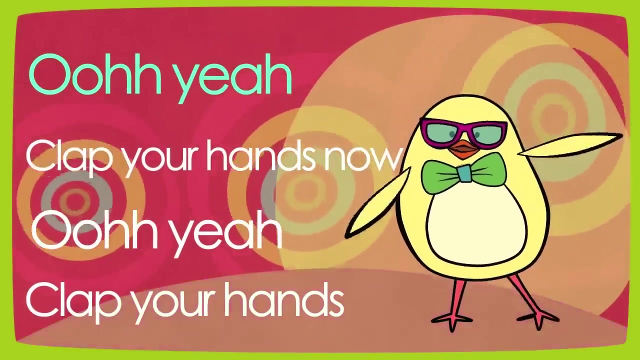 9 and 10: Raise your hands. Oh yeah, sing with me now. Oh yeah, sing with me. Oh yeah, sing with me now. Oh yeah, sing with me. Oh yeah, clap your hands now. Oh yeah, clap your hands. Oh yeah, clap your hands now. 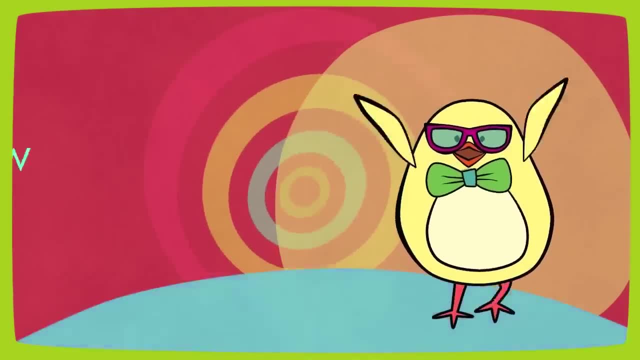 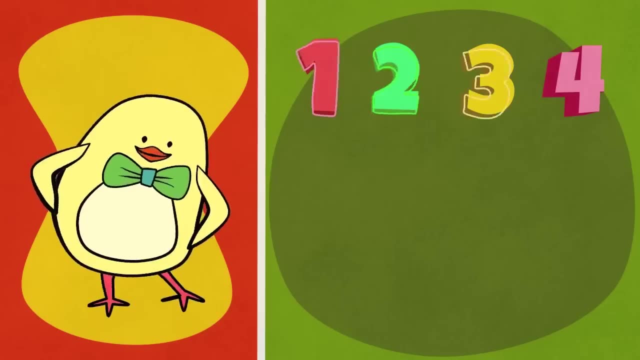 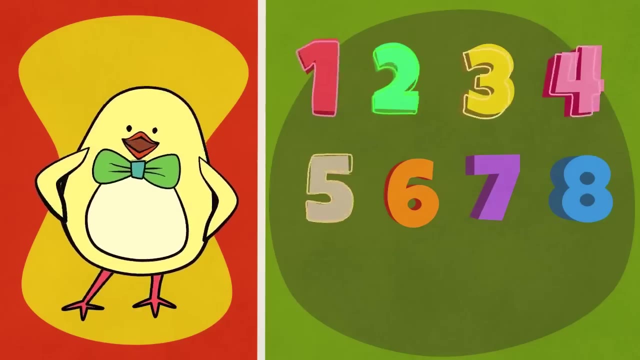 Oh yeah, clap your hands: 1,, 2,, 3, 4. 1, 2,, 3,, 4, 5,, 6,, 7,, 8, 5, 6,, 7,, 8, 9 and 10.